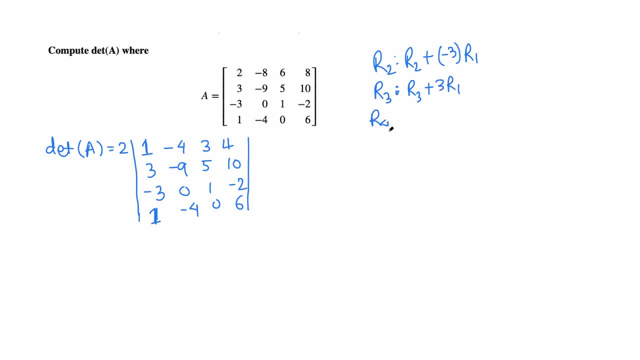 And now we have r1.. Okay, now let's make this 0 as well, so row 3 such that row 3 plus negative 3, so multiply by 3, 3r1.. for r4, this is 1, so do not multiply by anything to this corresponding row. so 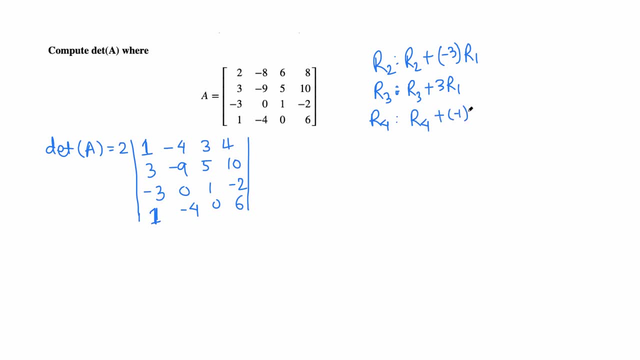 r4 and plus negative 1 r1. so we are doing these three things. so this determinant is equal to 2 outside and we are not doing anything to the first row: 1 negative, 4, 3, 4. now this is 3 minus 3, 0 negative, 9 plus 12, 3, 5 minus 9 negative. 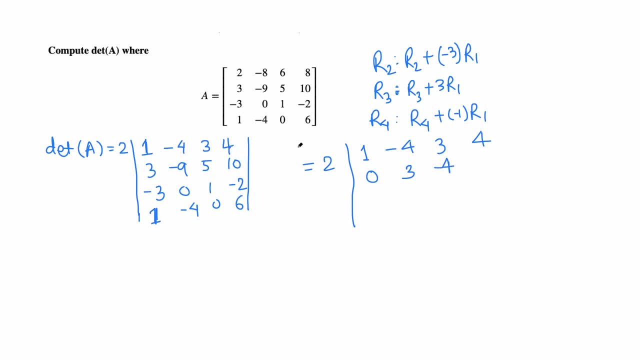 4, 10 minus 12. that's negative 2. in the same way, r3: negative: 3 plus 3: 0, 0 minus 12. negative 12. 1 plus 9, 10. negative 2 plus 12. okay, that's 10 for r4: 1 plus negative 1: 0. 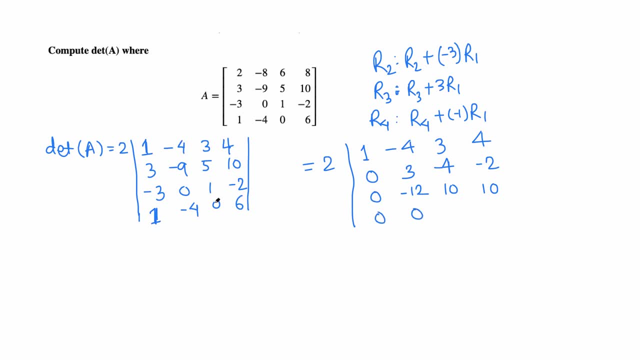 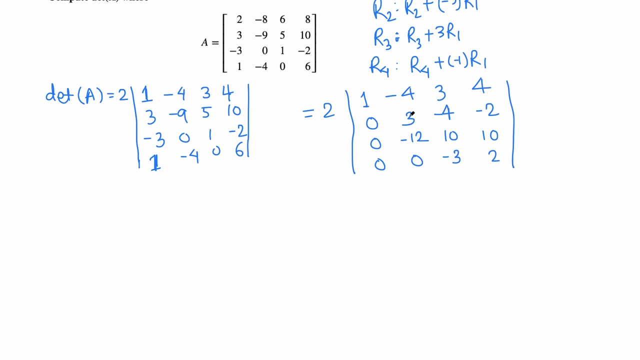 negative 4 plus 4, 0, 0 minus 3. negative 3: 6 minus 4: 2. okay, now, next, we want to make this 1, ok, ok, ok, ok, ok, ok, we're gonna make this 1 and 0 here and 0 here. we don't have to make this 1, but. 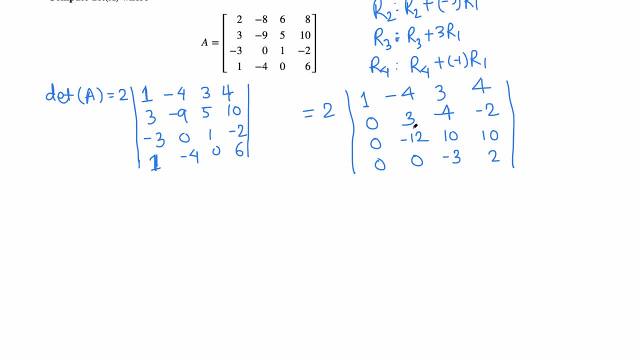 that might help us to get this 0, but this is kind of negative 12 already, so we don't have to make this one. ok, this is easy, so let's do work on r3. so r3 plus so negative 12. let's multiply r2 by. 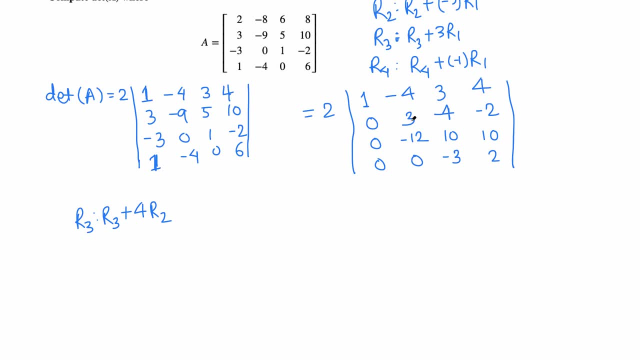 plus, so negative 12. let's multiply r2 by plus, so negative 12. let's multiply r2 by 4, 4 r2, so this becomes plus 12 negative 12: 4, 4 r2, so this becomes plus 12 negative 12. 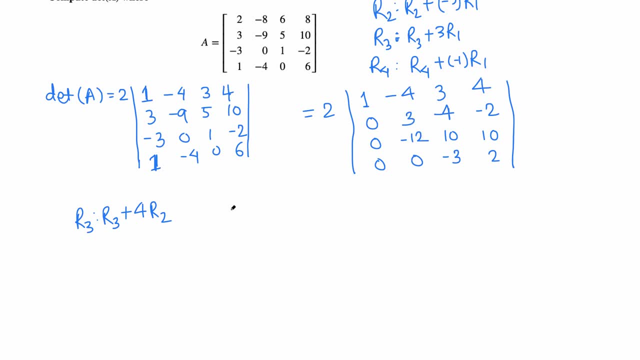 4, 4 r2. so this becomes plus 12, negative 12 plus 12: 0. ok, so we don't have to make plus 12: 0. ok, so we don't have to make plus 12: 0. ok, so we don't have to make this one. so this is 2 and not doing. 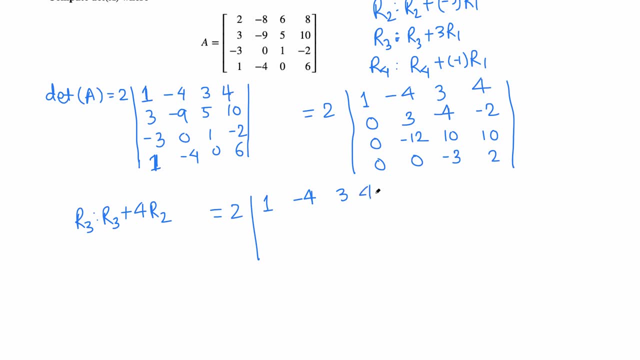 this one. so this is 2 and not doing this one. so this is 2 and not doing anything on r1: 1 negative, 4, 3, 4. not doing anything on r1: 1 negative, 4, 3, 4. not doing anything on r1: 1 negative, 4, 3, 4. not doing anything on r2: 0, 3 negative, 4, negative, 2. 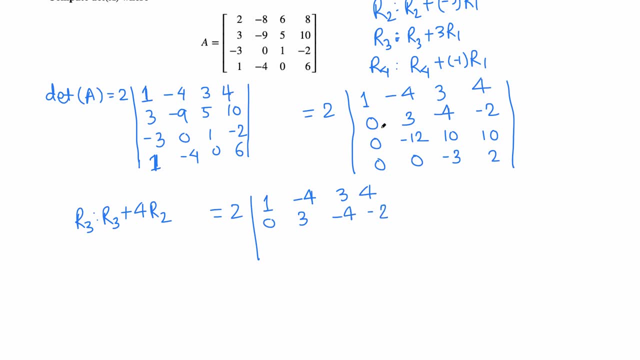 anything on r2: 0, 3 negative, 4, negative, 2. anything on r2: 0, 3 negative, 4, negative, 2. now the root. so we are using r2 right now the root, so we are using r2. right now the root, so we are using r2 right: zero, 10 plus negative, 16, negative, 6, 10. 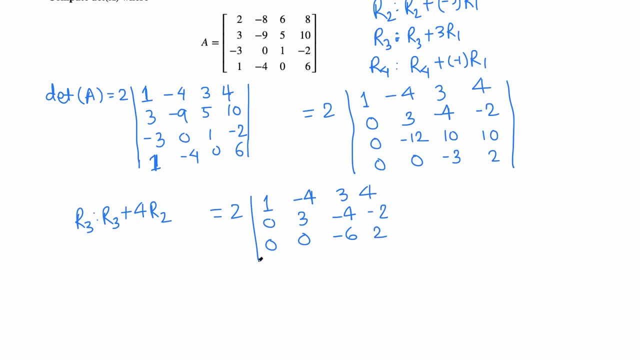 zero, 10 plus negative: 16. negative: 6: 10. zero, 10 plus negative, 16. negative, 6, 10 plus negative: 8, that's 2, and the last plus negative: 8, that's 2 and the last plus negative: 8, that's 2. and the last row is 0: 0 negative: 3: 2. ok, we are. 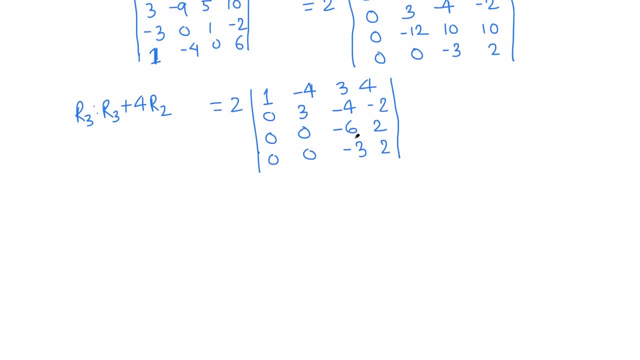 row is 0: 0 negative- 3, 2. ok, we are. row is 0: 0 negative- 3, 2. ok, we are almost there. so as soon as we make this almost there, so as soon as we make this almost there, so as soon as we make this element 0, then we have a upper. 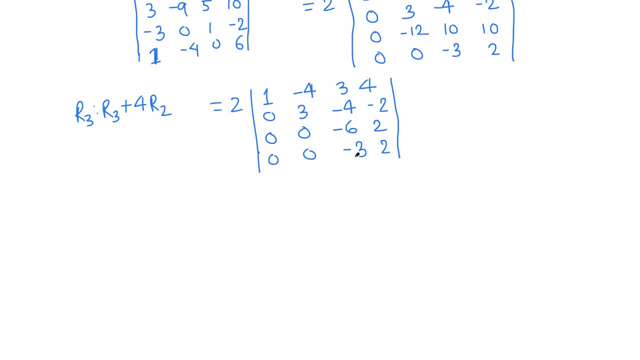 element 0, then we have a upper element 0, then we have a upper triangular matrix determinant. ok, so to triangular matrix determinant. ok, so to triangular matrix determinant. ok, so to make this 0. we can use this. we need to make this 0. we can use this. we need to. 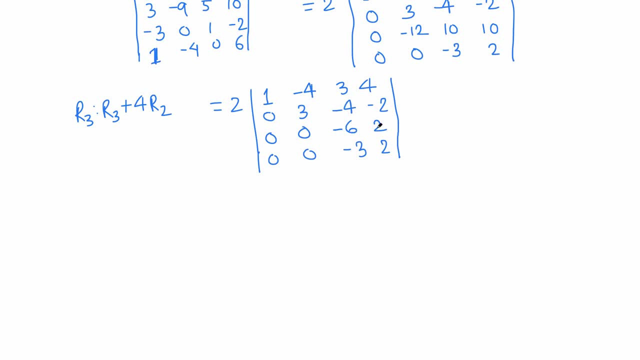 make this: 0. we can use this. we need to use this. ok, don't use this any other. use this. ok, don't use this any other. use this: ok, don't use this any other. negative 6 and 2: we can factor something. negative 6 and 2: we can factor something. 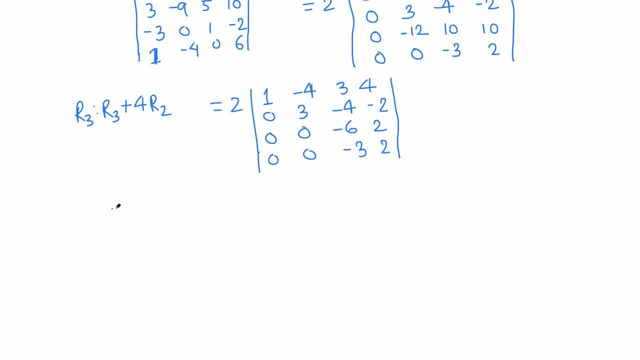 negative 6 and 2. we can factor something out from r4. you can factor 2: this 2 is out from r4. you can factor 2: this 2 is out from r4. you can factor 2: this 2 is already there. we can factor negative 2. 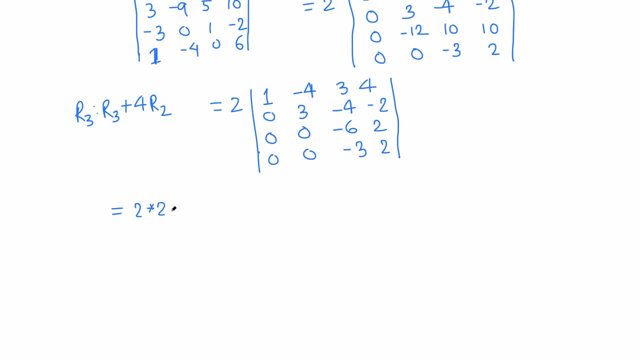 already there, we can factor negative 2. already there, we can factor negative 2 out or just 2, doesn't matter, just 2 and out or just 2, doesn't matter, just 2 and out or just 2, doesn't matter, just 2. and no change on r1. no change on r2. 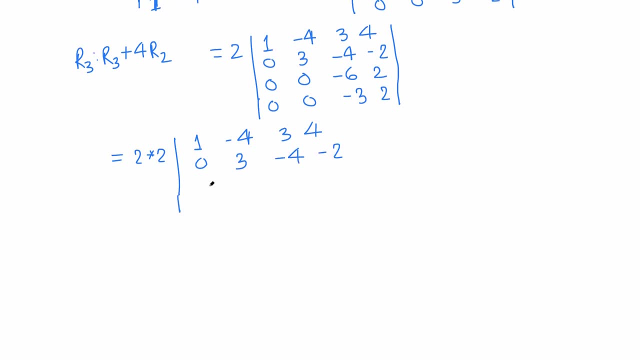 no change on r1. no change on r2, no change on r2. so when we factor 2 out, this is 0, 0. so when we factor 2 out, this is 0, 0. so when we factor 2 out, this is 0, 0 negative 3, 1, 0, 0 negative 3, 2. now we make: 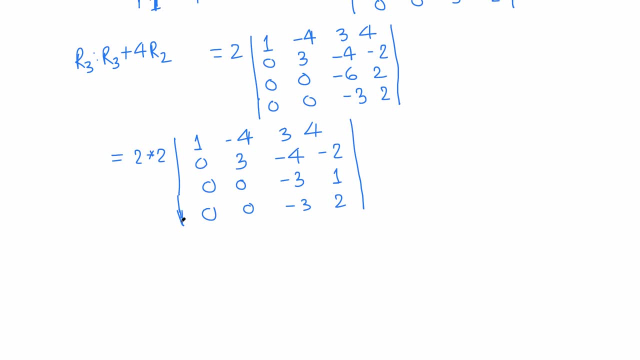 negative 3 1, 0, 0. negative 3, 2. now we make negative 3 1, 0, 0. negative 3, 2. now we make this element 0, that's on the r4. so this element 0, that's on the r4. so 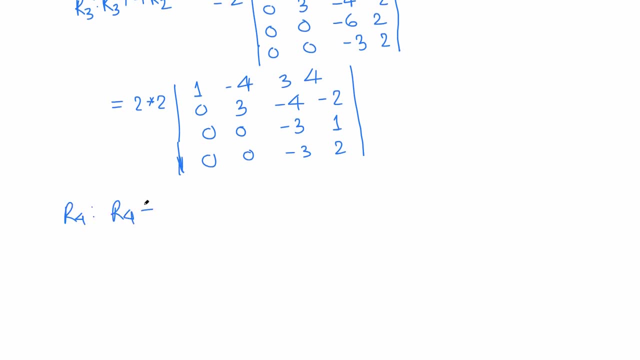 this element 0, that's on the r4. so let's do that. so r4, so r4 plus. do not let's do that. so r4, so r4 plus, do not, let's do that. so r4, so r4 plus. do not multiply by anything here: r4 plus. 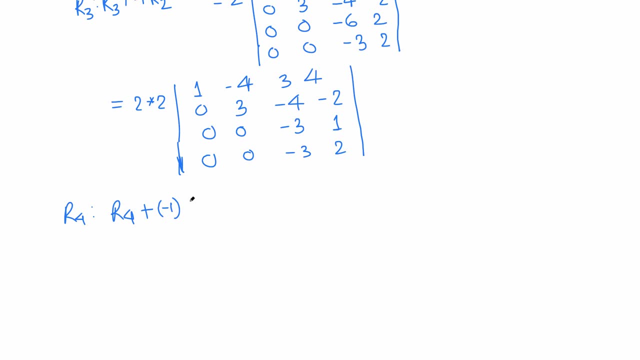 multiply by anything here: r4 plus. multiply by anything here: r4 plus negative: 3. let's multiply by negative 1: negative, 3. let's multiply by negative 1, negative 3. let's multiply by negative: 1, 2, r3. okay, we got. 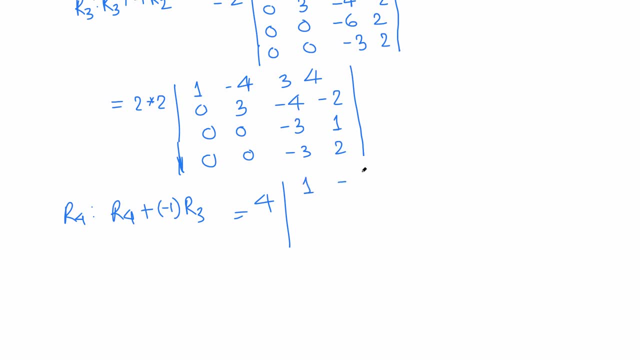 2 r3. okay, we got 2 r3. okay, we got 2 times 2- 4 outside 1 negative: 4 3 4 0 3. 2 times 2- 4 outside 1 negative 4 3 4 0 3. 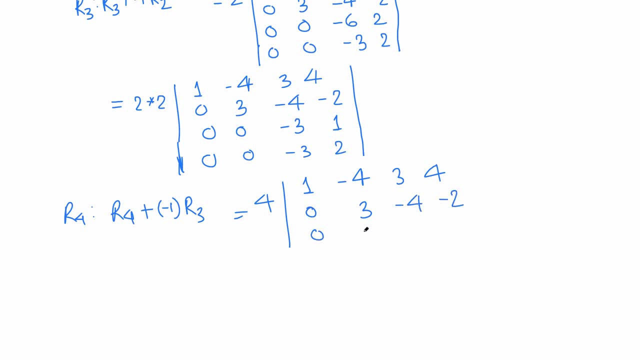 2 times: 2, 4 outside 1 negative 4, 3, 4 0, 3 negative, 4 negative 2 0 0 negative, 3 1 negative, 4 negative, 2, 0 0 negative, 3, 1. 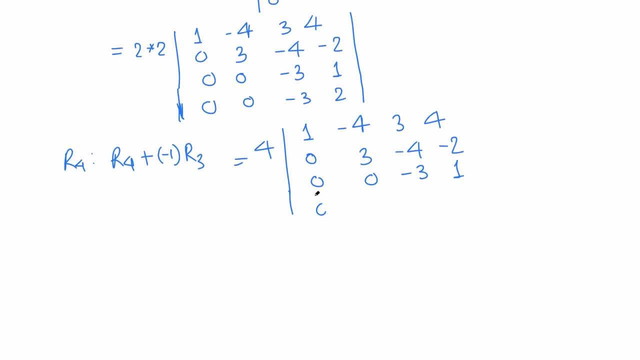 negative 4 negative 2, 0, 0 negative, 3, 1. and then now 0 just 0, 0, 3 negative, 3 plus. and then now 0 just 0, 0, 3 negative, 3 plus. and then now 0 just 0, 0, 3 negative, 3 plus. positive 3, 0, 2 plus, negative 1 just 1.